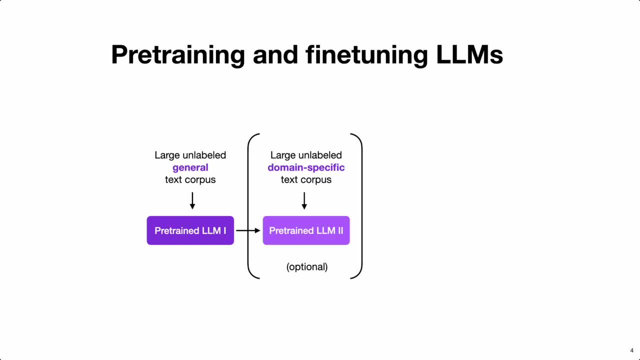 And then if we have a specific problem, a domain specific problem, for example in the medical domains or finance, we might want to train the LLM further on domain specific data. if we have such data, then once the LLM is ready, we can either use the pre trained LLM with in context. 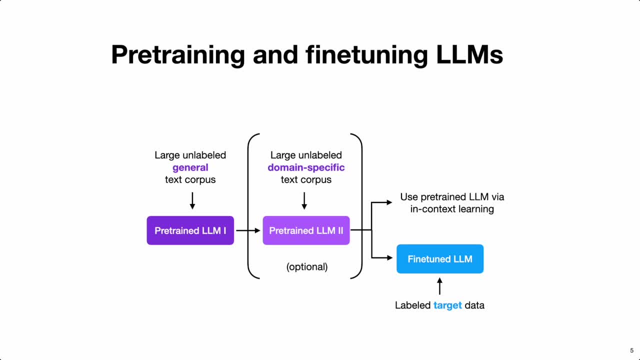 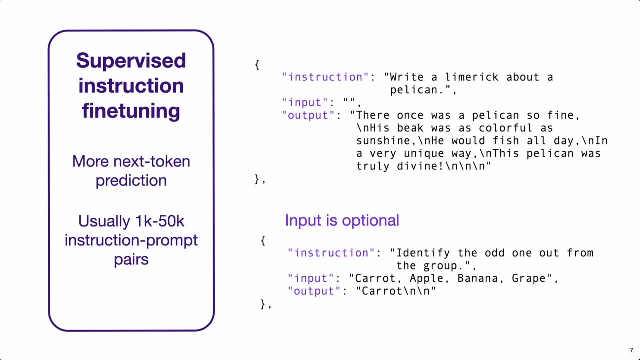 learning capabilities, where we ask questions, provide examples in the context, or we might want to train the LLM with in context learning capabilities. So that's what the talk here focuses on: better instruction, fine tuning. So in this particular talk I only used supervised instruction. 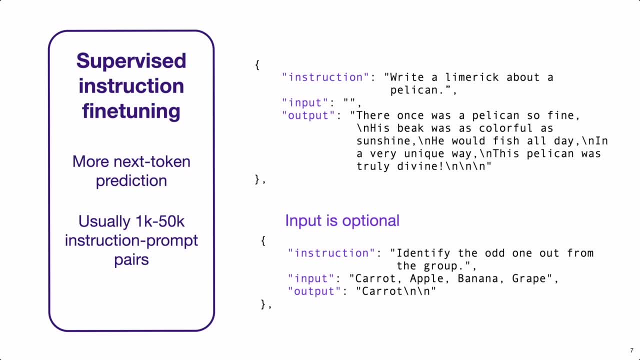 fine tuning. I know there are different ways of instruction fine tuning, including reinforcement, learning with human feedback and direct preference, optimization and so forth, But these are future problems, So here we focus on supervised instruction fine tuning, where we have a data set consisting of the instruction. 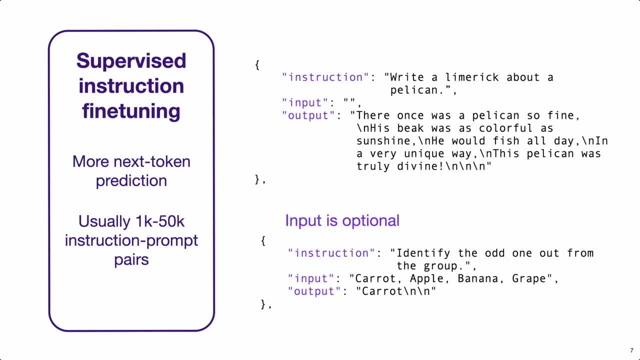 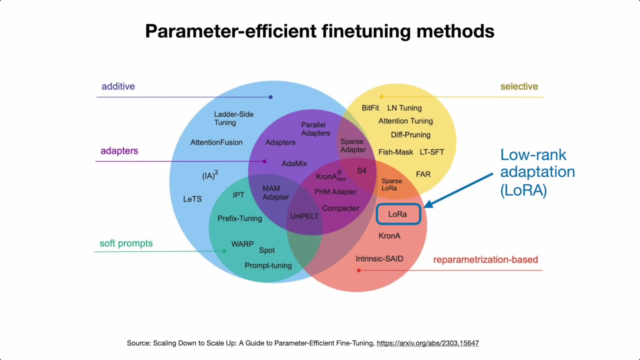 and the LLM task is to generate the output. Usually it's a next token prediction task where the LLM learns to generate one word at a time for the output, So to make this more efficient. because the LLMs are large people, over the years developed many 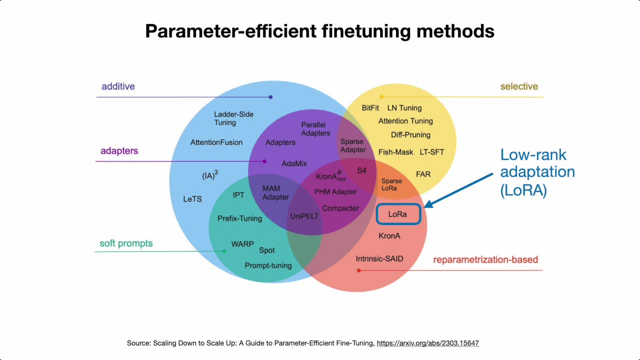 many different techniques And this is a nice survey here where most of the popular techniques for parameter efficient fine tunes fine tuning are visualized. But by far, far the most popular method is a low rank adaptation, Laura, And that's probably because it's very nice and elegant and works. 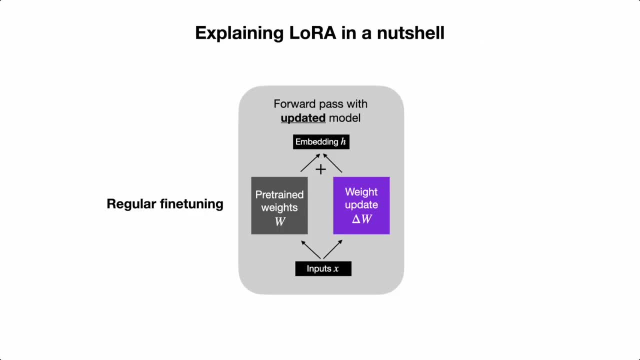 well in practice. So how does Laura work? before I dive more into the experiments, What is Laura and how does it work? So to explain that with a, let's say, a few slides, because we only have so much time here. So imagine you have the regular. 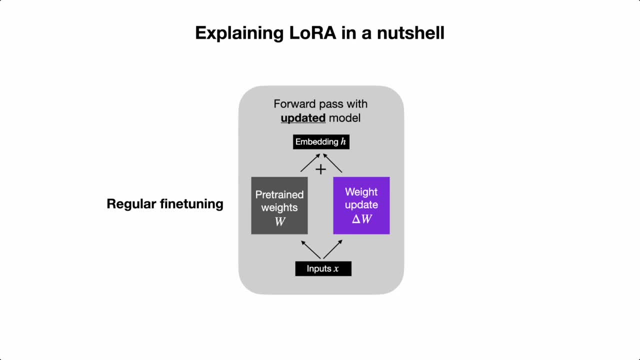 fine tuning setup where you want to update the pre trained weights here. I'm writing this separately, where you have the pre trained late awaits and on the left hand side and you have the weight update here on the right hand side And I'm writing: 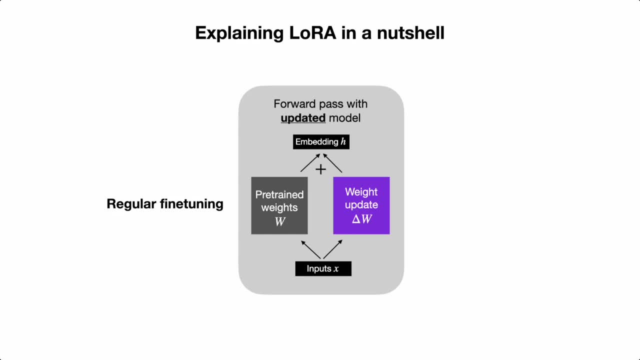 it like this, so that I can then show you how Laura relates to that. So imagine you saved the weight update separately, as a separate matrix, instead of just applying it back to the pre trained weights. then you can think of Laura as a low rank. 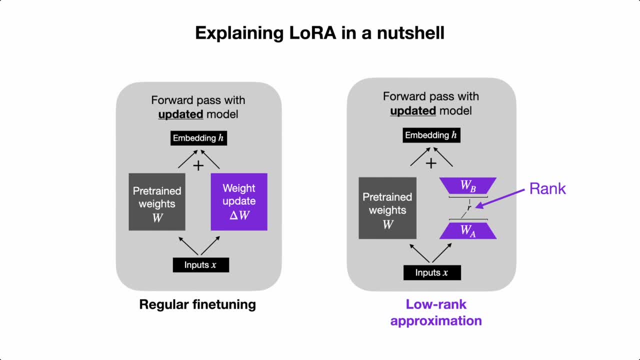 approximation or decomposition of that weight matrix. So instead of on the left hand side learning this full weight update matrix is in regular fine tuning, what Laura is doing it's learning these two smaller matrices And the trick here is that we have this rank And we can choose a very small rank for these. 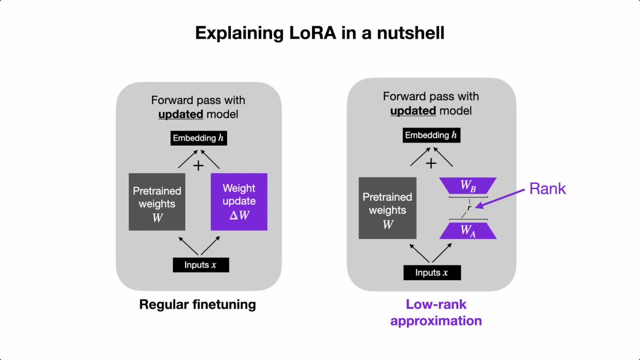 matrices to save a lot of parameters which will make the training more efficient. So, for example, consider on the left hand side we have 5000 times 1000 parameters, for example, that would be 5 million parameters in that matrix in. 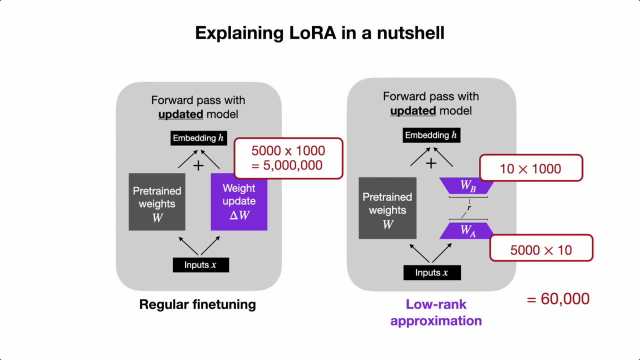 total. And on the right hand side, if we have a rank of 10, we would have 10 times 1000, or let's say 5000 times 10 plus 10 times 1000, which is 60,000 parameters, which is much less. 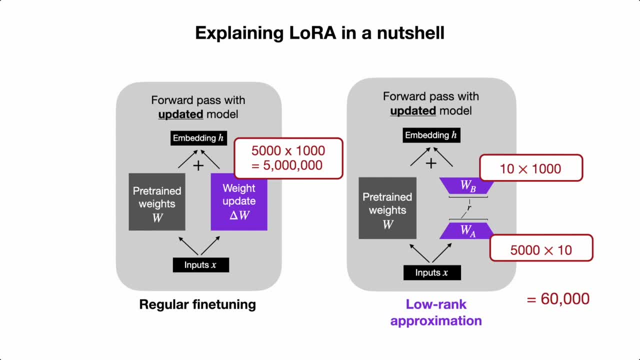 than 5 million, Of course, are. the rank is a hyper parameter, But if we choose a small, are like 10 here- then we can save a lot of parameters And the idea is that with this role, a low rank decomposition, we can approximate the results of the 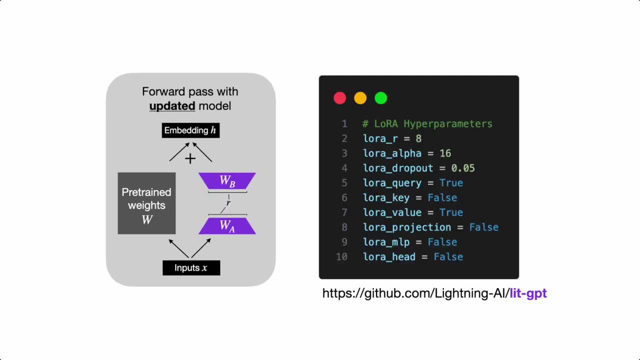 full weight update here. Now. in practice, however, there are lots of settings. So when we are using Laura, there are lots of little little tweaks we can do. there are lots of parameters that come with Laura, for example, for which layers we want to apply Laura, or there's. 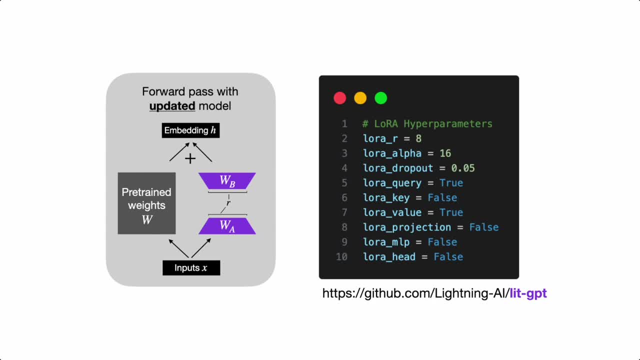 also the scaling factor, alpha and so forth. So for now I will start with default parameters that we have chosen in lit GPT. So this is only activating, Laura for a few layers in this LLM. So the query, key and value and so forth, they refer to the layers. 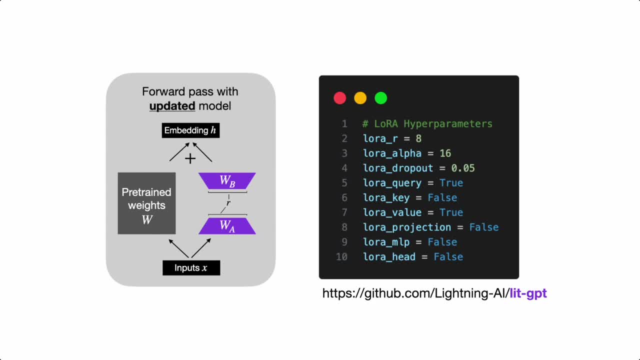 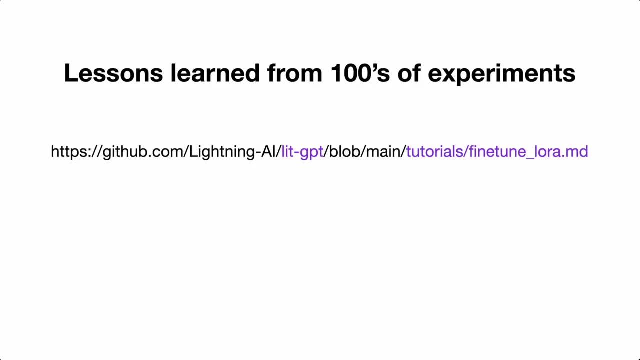 in an LLM, the query key and value of attention head, And so we are only enabling it here for a few, and later we will change the settings. So I wanted to share now a few of the results I got from running hundreds, if not 1000s, of experiments And if 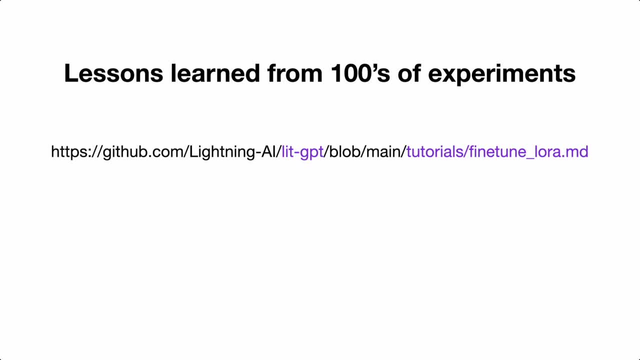 you're interested, there are also tutorials on GitHub. So I'm not showing any code here because it's a short talk, But if you want to get run Laura, fine, tuning yourself, you can find the tutorials here. So to start with one thing I found 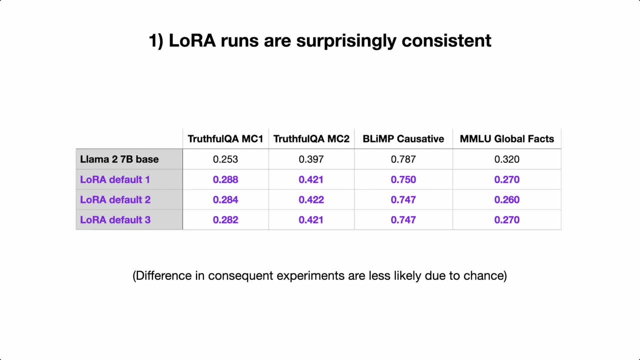 and I found very nice is that, Laura, runs are surprisingly consistent, which means when I was changing the hyper as the random seed, I found that the results were pretty consistent across runs, which is a good, good thing to have when you are running experiments. you know okay, these are approximately. 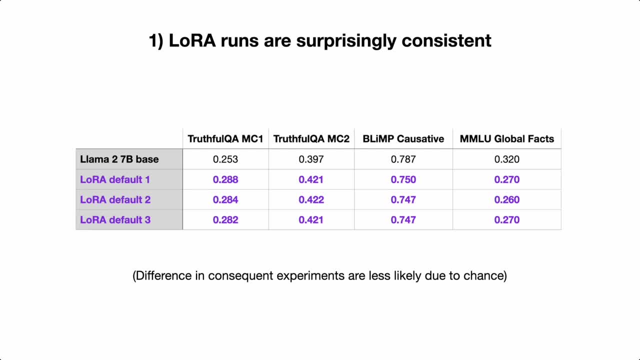 reproducible And it's. if you get some odd layers, it's less likely due to the random seed or due to the random seed. So if you've got a real kind of a high standard area, it's it's not always going to be do well. So I realized that if you're 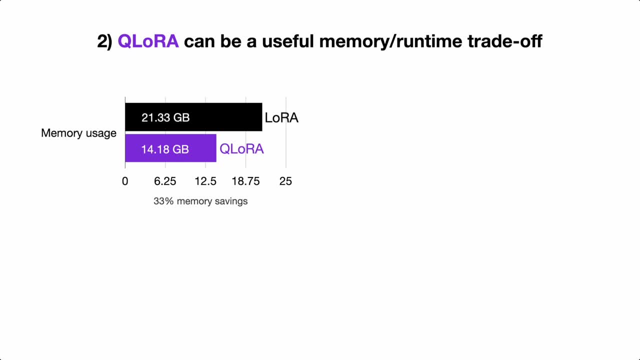 just trying to get a single queue chance. the other one was I was trying as hard as possible to save compute memory so that I can later on train larger LLMs on one GPU. So here I was doing experiments with a 7 billion Lamma to model. the reason is: 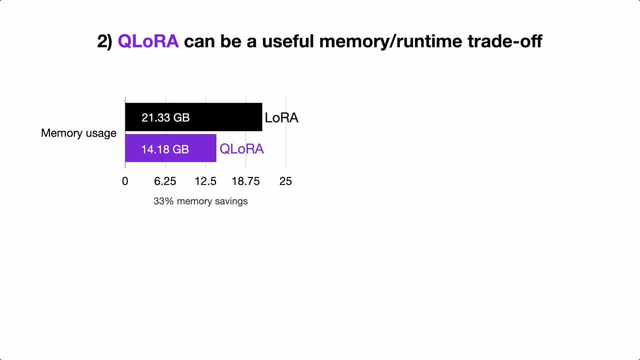 because I wanted to also later, compared to full fine tuning and I couldn't do or couldn't fit larger LLMs, I was able to save about seven gigabytes in this case. uh, 33% of the memory, which is really nice, but yeah, in practice, um be aware, if you use quantized Laura, because of 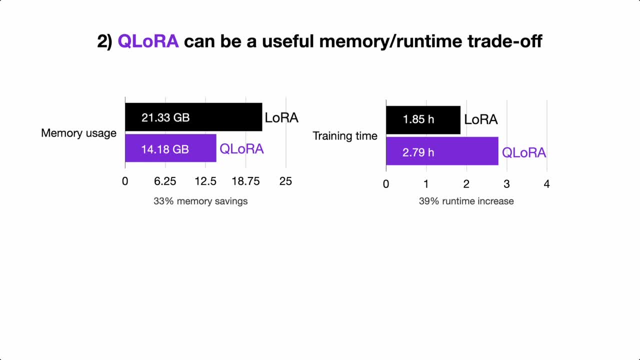 the additional quantization and de-quantization steps, there's an additional cost of computation costs. So in this case it was a 39% runtime increase. in practice, personally, I find it more useful to reduce memory because I usually can wait a few more hours, let's say for run things. 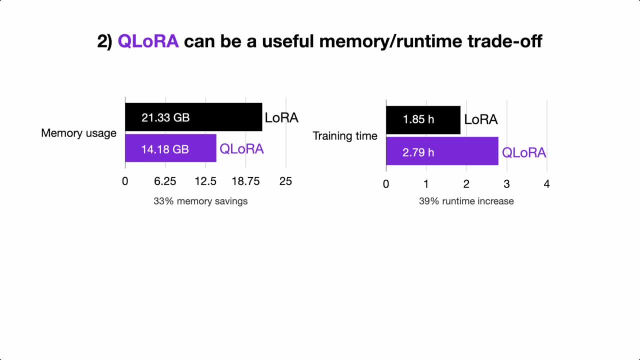 overnight. But if I run out of memory, it's usually the distinction between being able to run something on the GPU or not. So I kind of like the memory savings here. uh, when it came to the results on the benchmarks, I tested it on. uh, using Q. Laura, I would say it's plus minus zero on one task. 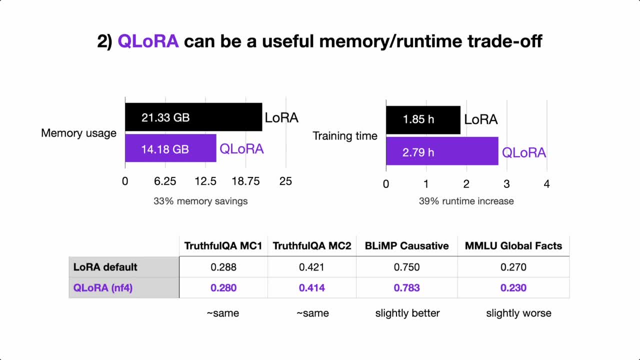 It was slightly better than one task. It was slightly worse. So I wouldn't say one is necessarily universally better than the other. I would say it's like plus minus zero, depending on What you're looking at here on. the next experiment was um. I wanted to save even more memory. 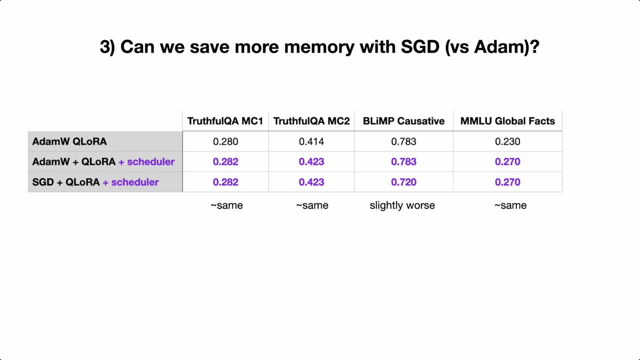 and I was wondering: can I swap Adam with SGD? because Adam saves two additional parameters for each model, parameter which can be expensive if you have large models. So I was wondering: uh, can I save memory if I just change Adam to SGD? 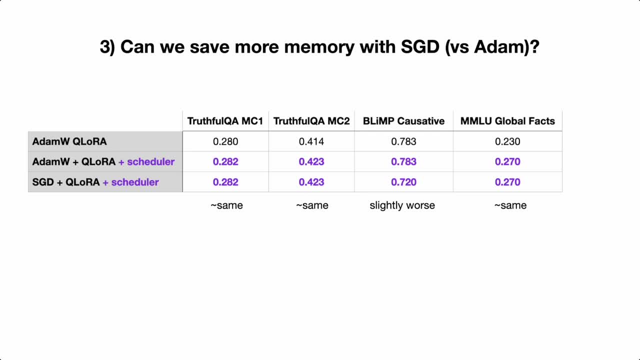 So here I was also adding a scheduler, because without a scheduler I was not able to get good SGD results. But yeah, the bottom line is that, Uh, SGD was slightly worse on one of the benchmarks compared- um, yeah, compared to. 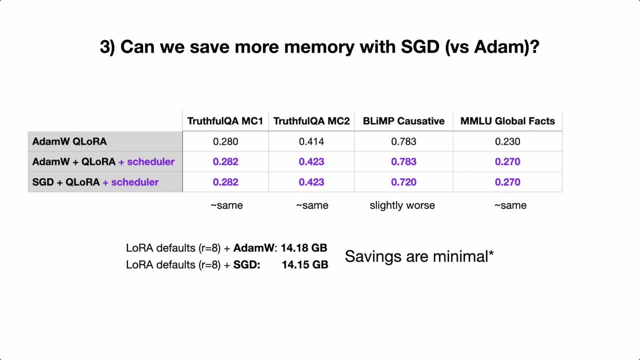 Adam Uh. however, unfortunately the memory savings were minimal and that is because we only had, like uh, about 4 million trainable parameters here, because we were using a small rank. However, your mileage may vary if you use a larger rank. more on that later. 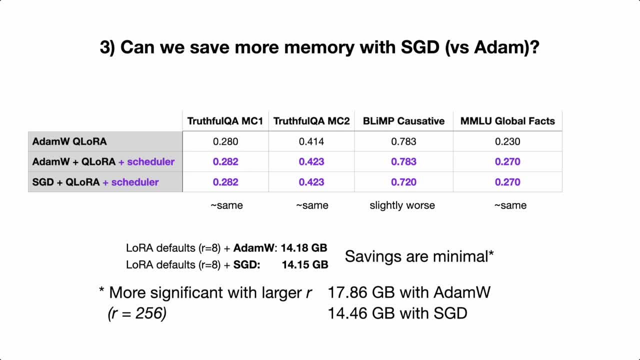 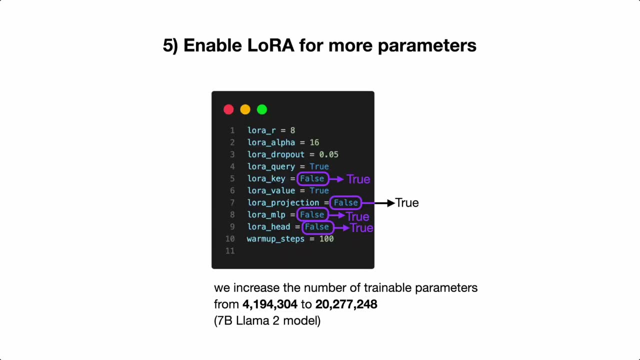 But for comparison, when I changed the rank to 256, I got about three gigabytes of savings, which can be actually significant. So if you are experimenting with larger ranks, yes, it is worthwhile thinking about replacing Adam with um SGD. 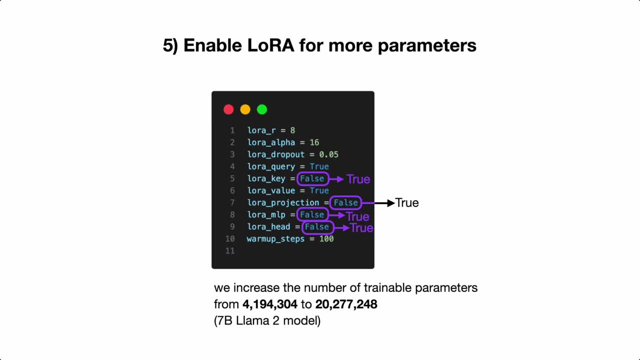 So what about these other parameters now, or hyper parameters now? So what if we enable Laura for more permit parameters in the network by activity or setting these hyper parameters to true? So if we do that, if we enable a Laura also for the key, the projection, the linear layers, 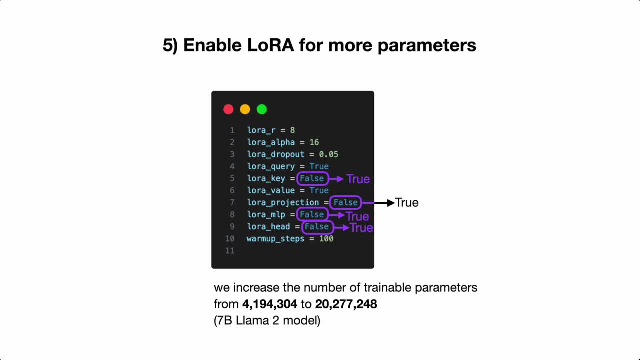 and the projection head. We increase the number of trainable parameters in that model from 4 million to 20 million. It's a five times increase. by what is the increase in terms of the performance? Um, I wanted to say also, by the way, this takes about three hours now. uh, it's using. 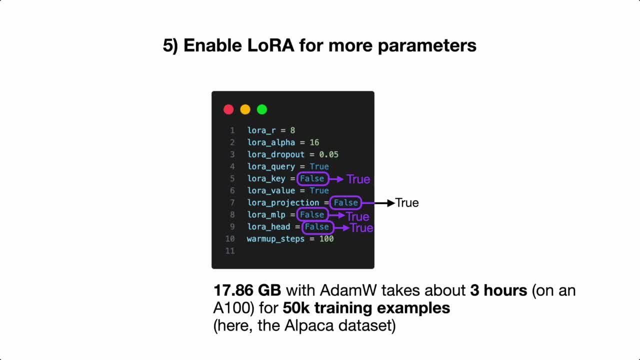 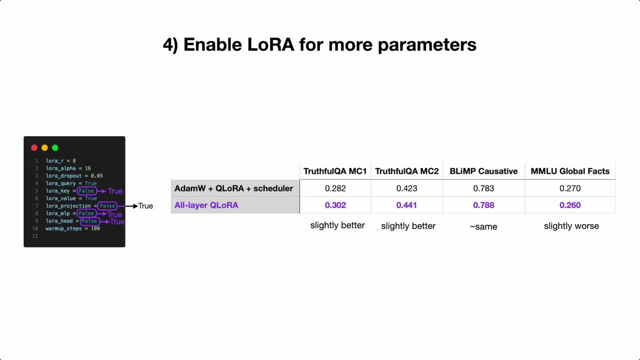 17,. uh, eight six gigabytes. before, we had something like 14 gigabytes. It's a three gigabyte increase. So if we do that, um, we can see that the results are slightly better. Um, except On one benchmark it's slightly worse, but overall I would say, yeah, it's a mixed bag. 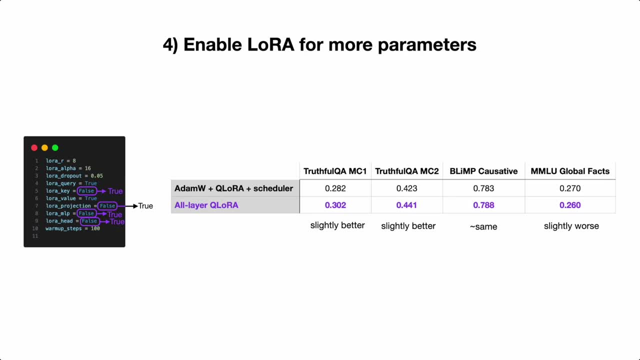 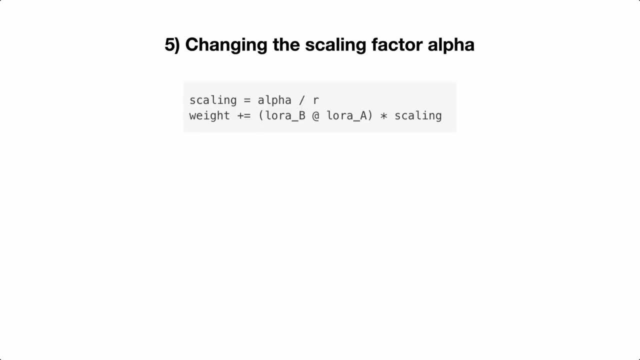 So just increasing the hyper parameters does not really bring us that much, given that we increased the number of parameters by a factor of five. So what can we do about that? So there is actually this um scaling factor alpha here that we can change. 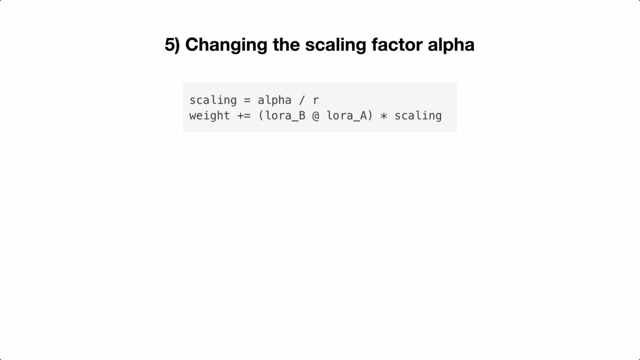 So the scaling factor determines how strong, let's say, or how much of the, the, the weight matrix, we add to the original weights. Like we are scaling the weight update here, It's it's kind of like a learning rate, if you will, except the learning rate is applied. 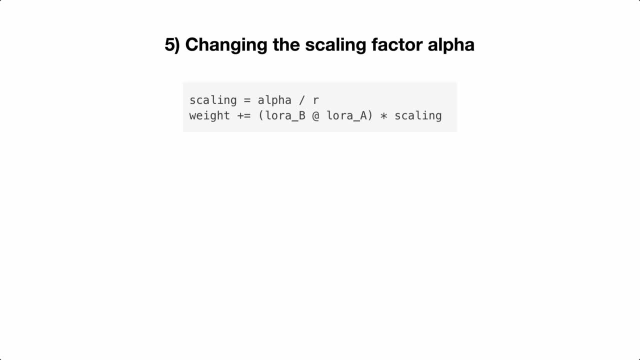 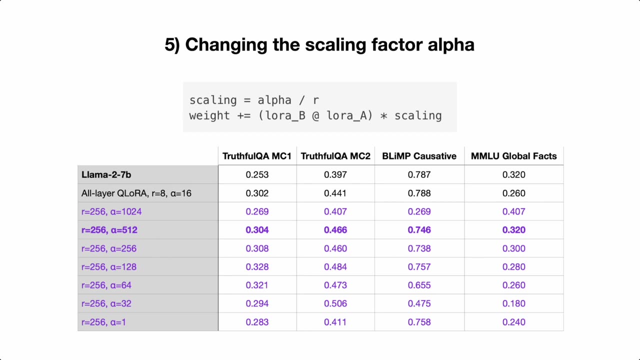 during the backward pass. by here, This is during the forward pass. So if we um change the rank and we changed the alpha, we get various different results. I'm showing you only the interesting ones, So I tried: smaller ours, larger ours. the R of 256 was performing best. 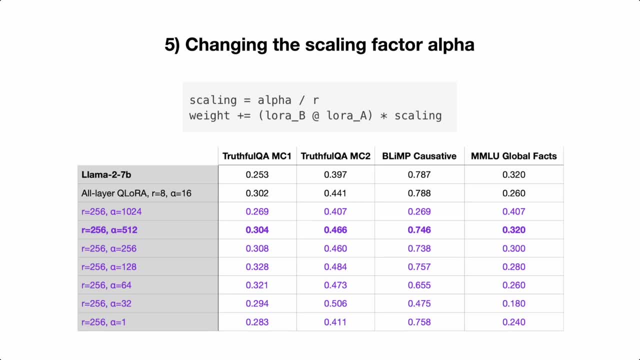 And I found that if you use an alpha of 500 to 12, which was about um alpha, two times the rank- then I usually- I would say roughly I- got the best results here. and you can see, on most benchmarks there's an increase, except on one of them there's a decrease. 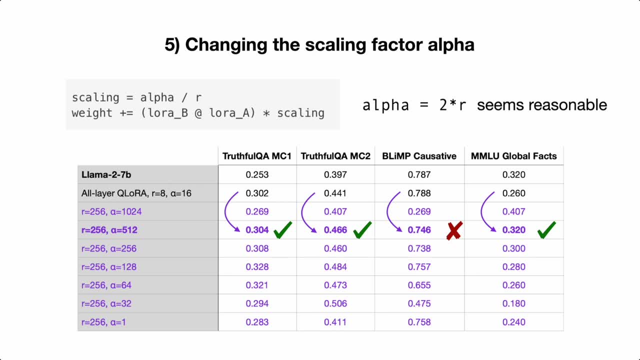 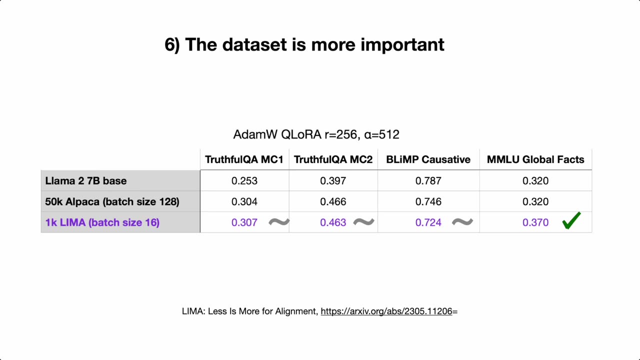 So again, it's, I would say, overall improved, but it is not um, not amazing, but this is what it is um. compared to the original llama model, It is much better, though I would say Okay, So, um, yeah, uh, last, uh, experiment is that also the data set is important. 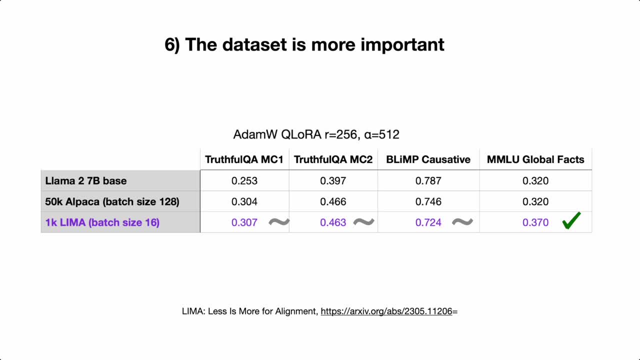 If you are experimenting with LLMs, I would say: don't just tune hyperparameters, also consider data sets. So here I did an additional experiment using a 50 times smaller data set and, surprise, surprise, I got actually better results with a smaller data set. uh, compared to the Alpaca data. 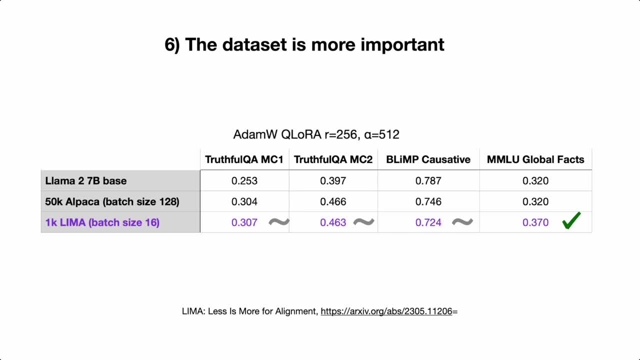 set. So here um, I also ran a lot of experiments and I found that are 256.. And 500 12 was also performing best, but I did have to change the batch size a bit um to get good results. 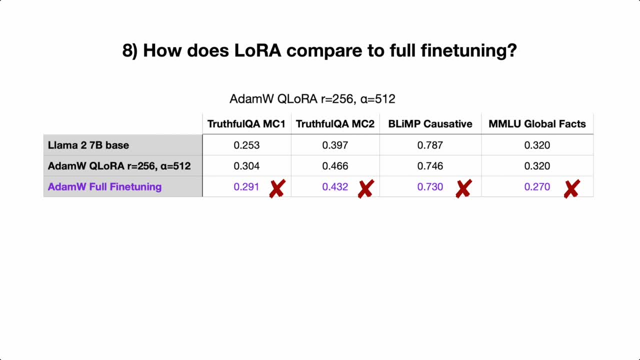 Um, lastly, for those who have questions about how does it compare to full fine tuning: a full fine tuning, to my surprise, was actually doing even worse, And so maybe it's the data set that was not very good to the Alpaca data set. 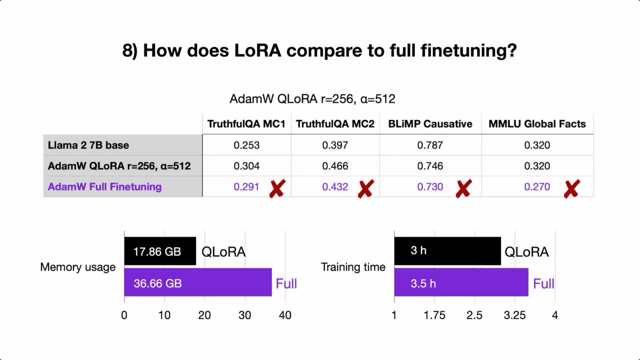 Um, so in that case, uh, full fine tuning was much more expensive, more than twice the memory consumption. Okay, So I think that the runtime was increased. So here, um, the bottom line is: yeah, um, QLora can be useful. but I would say also: